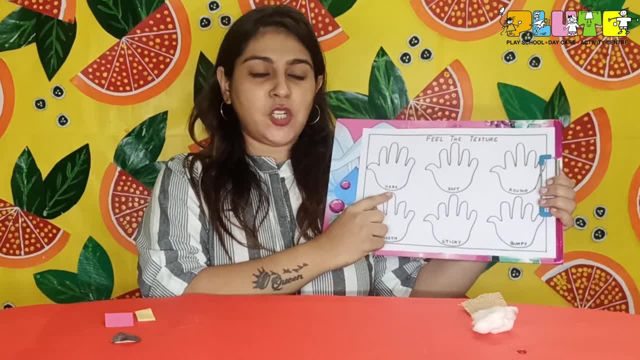 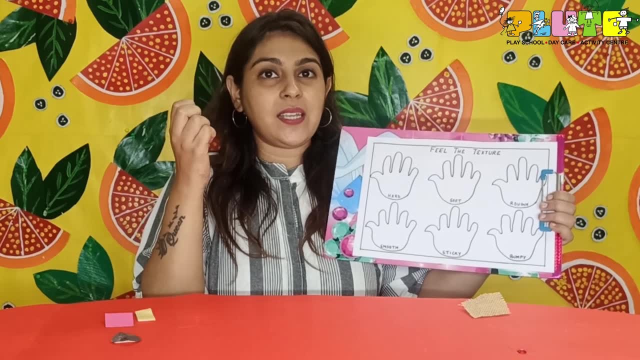 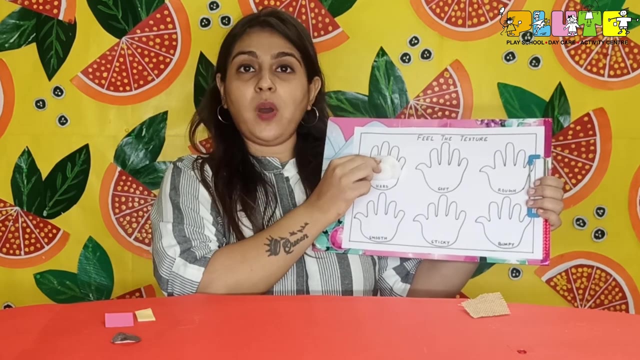 So let us find an object that is hard in nature. See, children, this is a cotton. I can easily squeeze it. Is it hard? No, it is very soft, isn't it? So I cannot place it over here. So let us find an object. 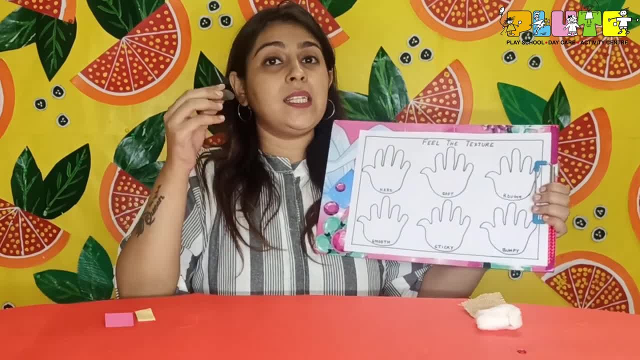 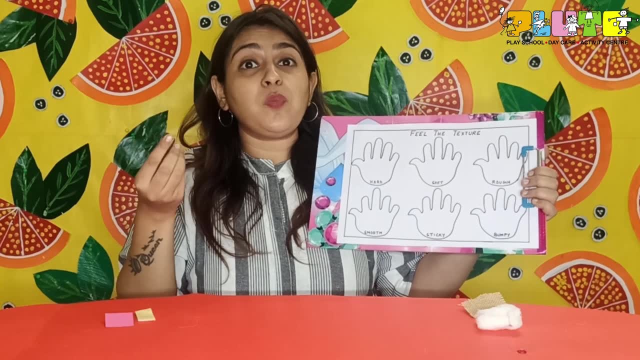 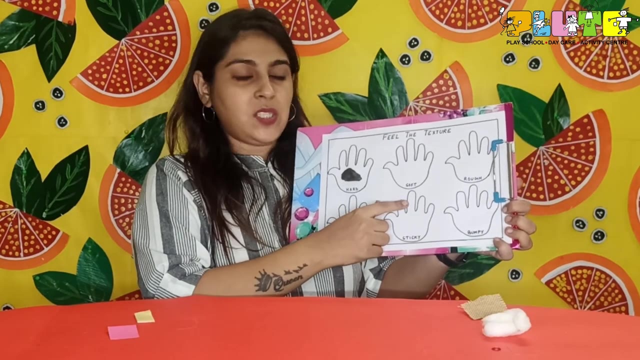 That is hard. This is a stone. Can I squeeze it? No. Can I bend it? No, It is very hard. So I am going to place this stone over here. See, let us see the next one. It is written soft. 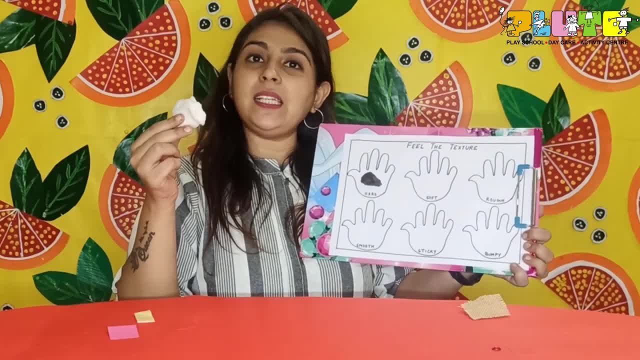 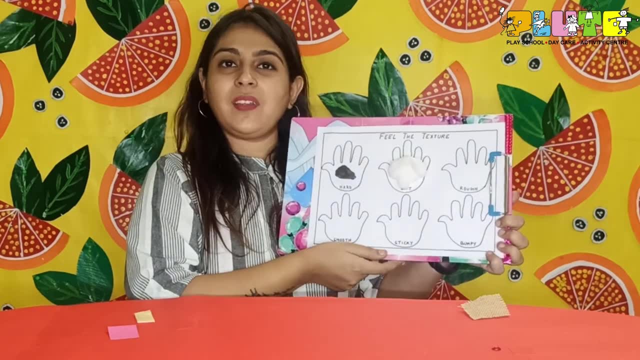 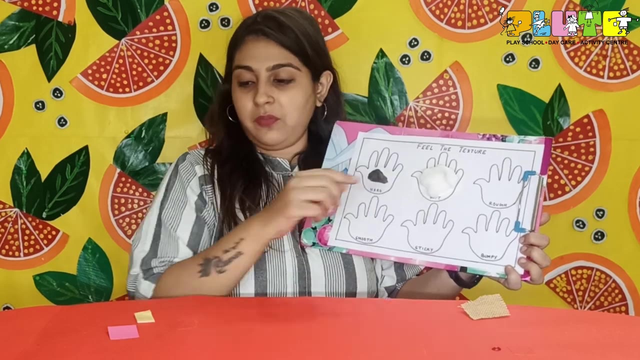 Children, we have already learnt that the cotton is soft. So I am going to take this cotton and stick it over here, Right? Let's see what is next. It is written rough. Let's see which object is rough. I have this paper in my hand. 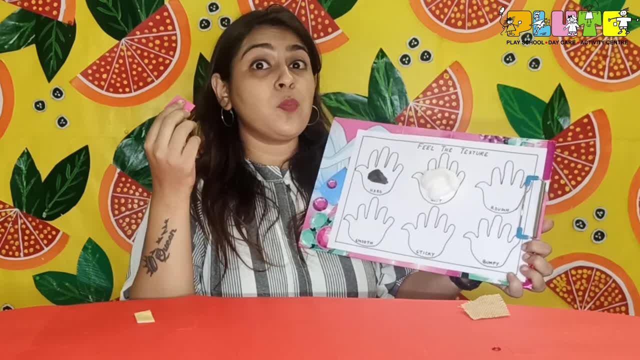 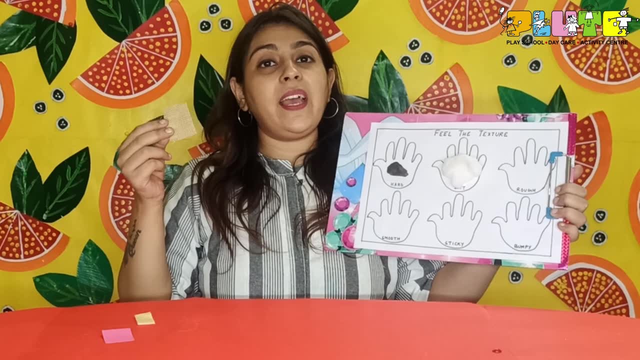 Is it rough? No, it is smooth. So let us find an object that is rough. See, children, I have a piece of jute cloth in my hand And when I try to feel the texture of it, it feels very rough. 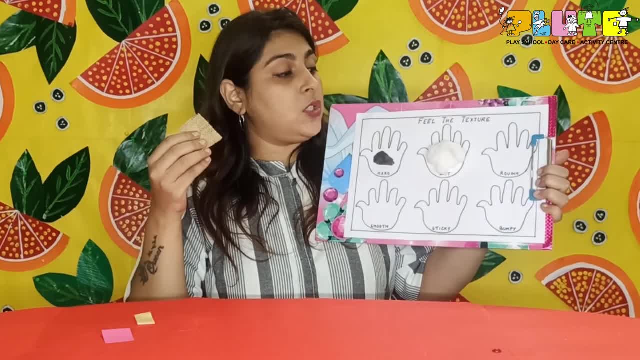 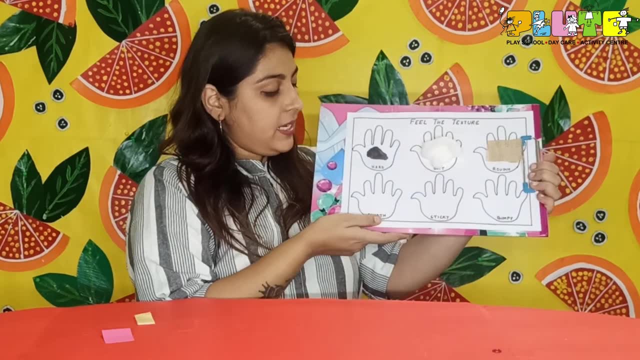 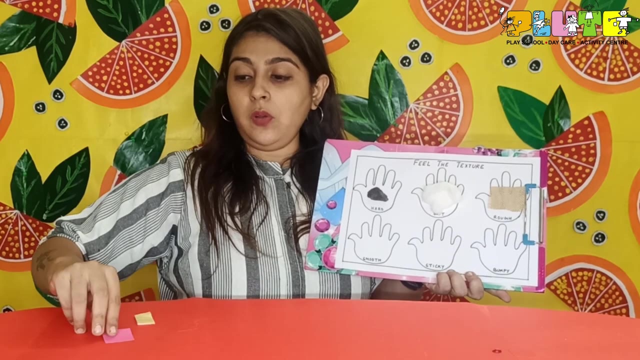 And when I try to feel the texture of it, it feels very rough. So I am going to take this and paste it over here, Because it feels rough. Let's see what is the other texture. It is saying smooth. So, children, earlier we got to know that this paper feels very smooth. 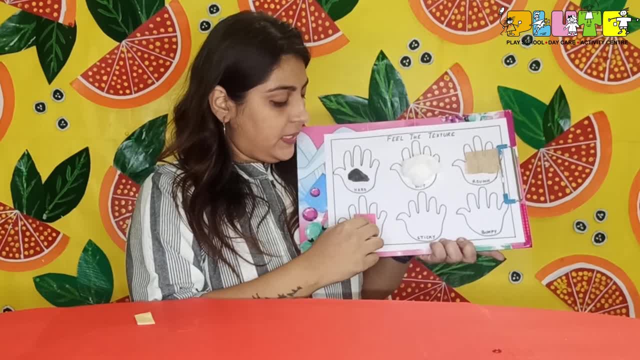 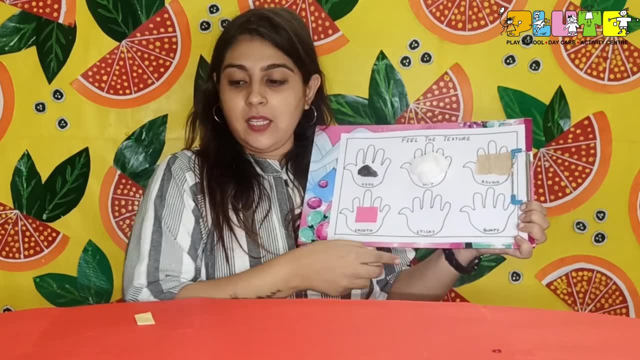 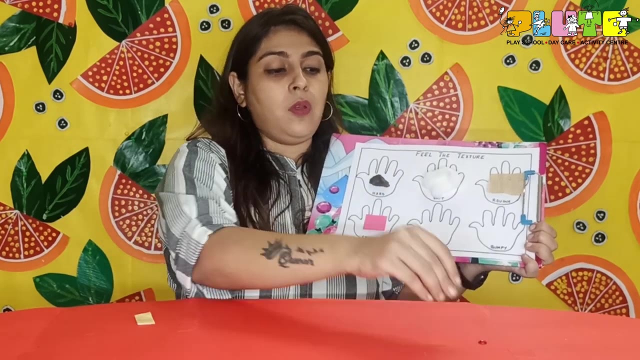 So we will take this piece of paper and paste it over here Like this Right. The next texture is sticky. So let's see which is sticky. So let's see which is sticky. Is this sticky? No, Is this sticky. 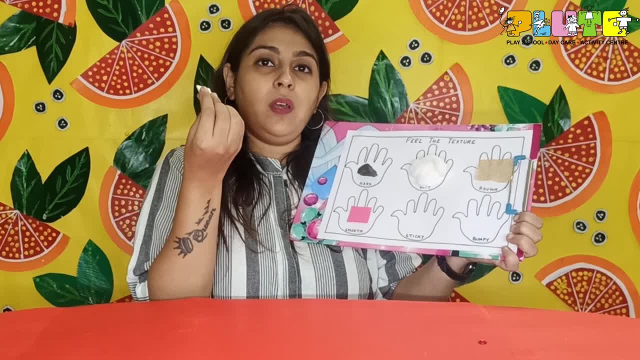 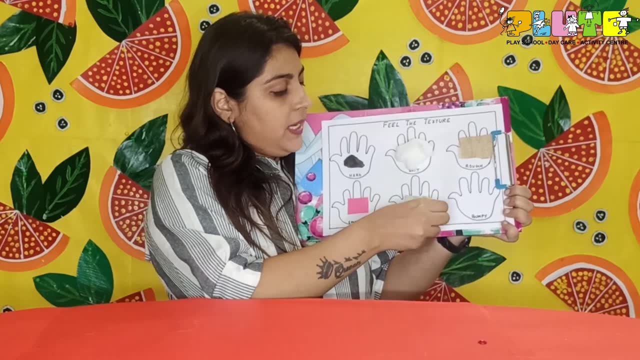 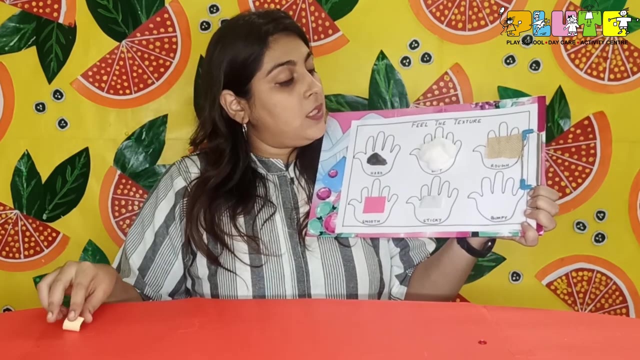 Yes, This sticky tape is sticky, from this side also and from the above also. See, When I remove the peel of this tape, it is sticky, Isn't it? Yes, So, lastly, it says bumpy. Yes, So, lastly, it says bumpy.